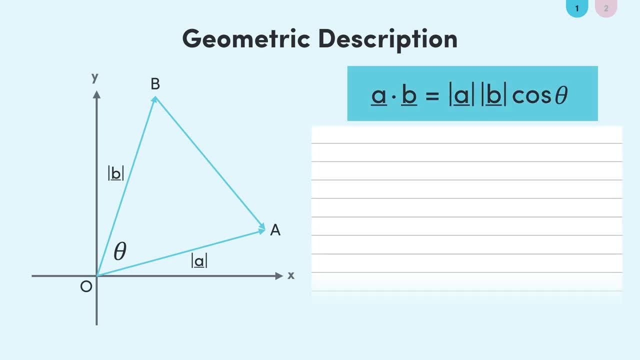 Now, what are the lengths of each side of our triangle? Well, the length of OA is just the magnitude of vector A, which is this: Similarly, the length of OB is the magnitude of vector B. What about BA? Well, BA, with the direction from vertex B to vertex A, is the same as the vector A minus B. 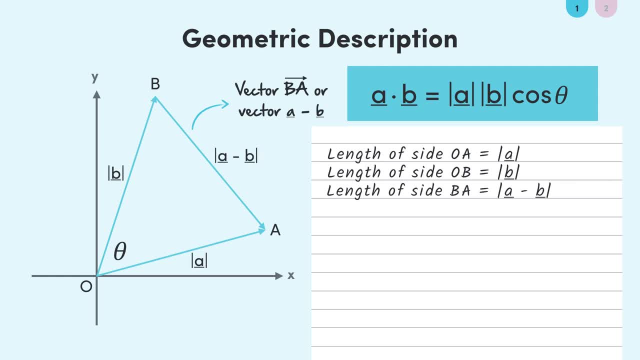 So the length of the side BA is just the magnitude of the vector A minus B. aka this Note, you could instead take the vector B minus A and the proof would be pretty much identical. So we have three side lengths of a triangle and an angle. 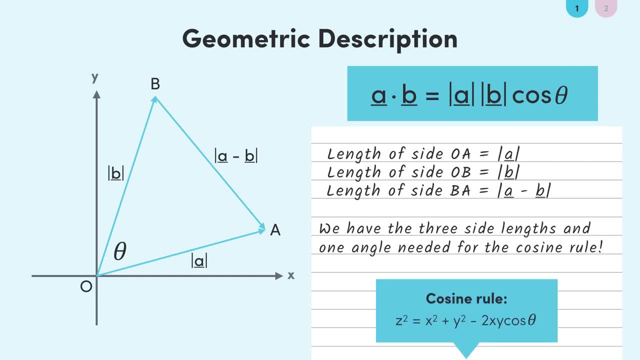 That's exactly what we need for the cosine rule. If we pull up the cosine rule for some general side lengths- x, y and z- then we can substitute in our side lengths. What I mean is letting x, y and z be these values. 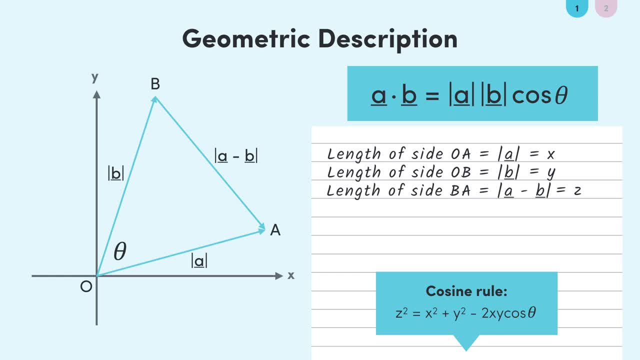 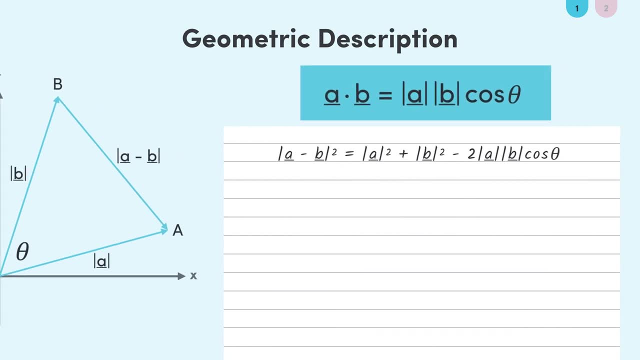 And, of course, our theta can stay as theta, as it is in the triangle OAB, Using the cosine rule, this is the expression we arrive at: Recall that the magnitude of a vector, a, is the square root of each entry. squared like so. 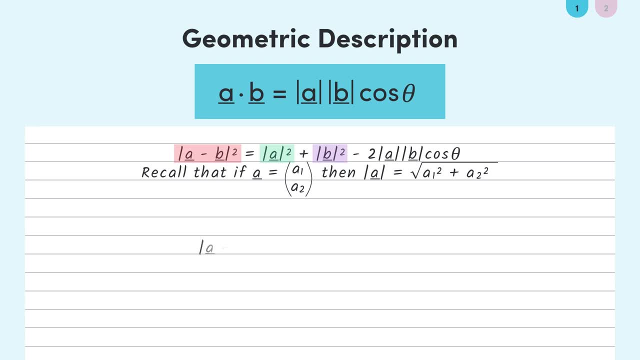 Notice, in our equation we have this quantity squared and these other similar terms. You can see the terms match up. Let's now substitute these into our equation. We've left this part of our equation untouched because- notice, it appears in our final formula. 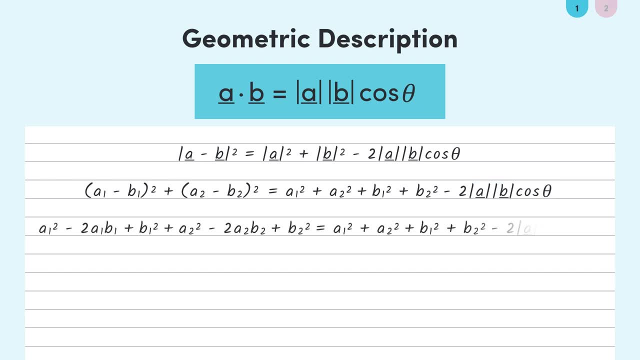 Now we can expand these perfect squares quite simply to arrive at this. There are plenty of like terms that cancel out on either side, so we can simplify to this. I hope you can sense we're very close to the formula we're trying to prove. 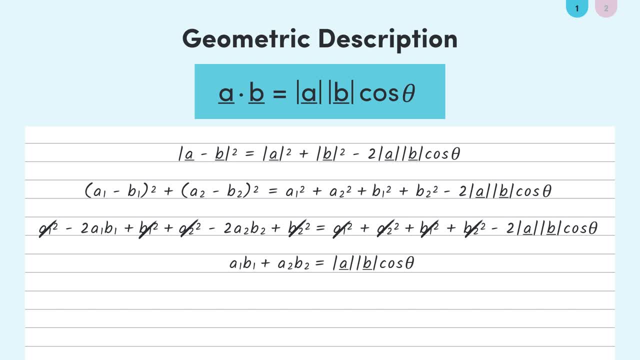 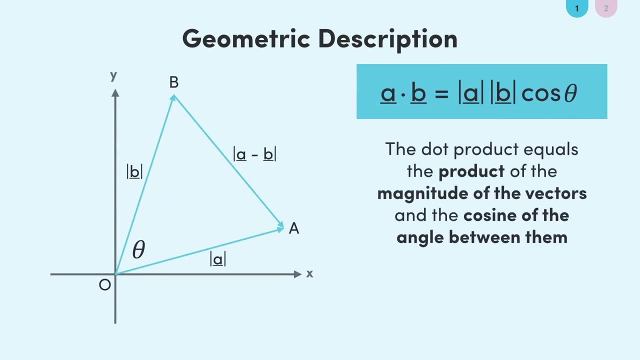 Dividing by negative two. and then the left-hand side is precisely what we defined the dot product between vectors a and b to be. So we're there. This is our formula for the dot product. from a more geometric view, This formula tells us that the dot product between a and b 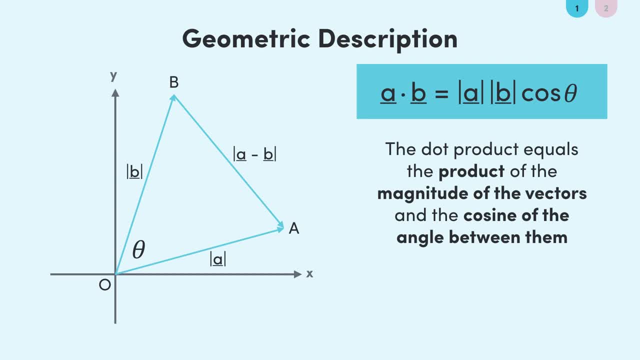 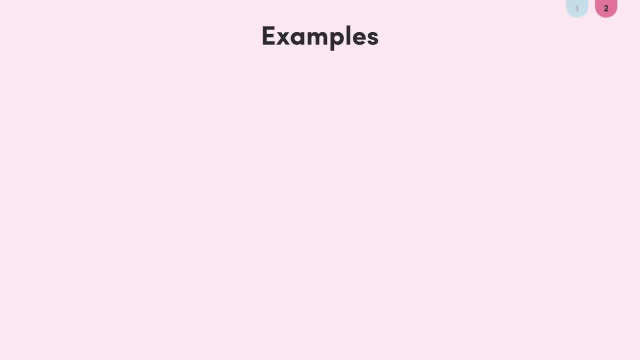 is the magnitude of the vectors and the cosine of the angle between them, or the angle between the vectors All multiplied together. You may be wondering what sort of questions will involve this formula, So let's look to a couple of examples now. Here's the first question.